They're moving more than water molecules in cooler air. That means they're less likely to condense out of the atmosphere and they end up hanging out in the air and making things feel all sticky. So temperature plays a big role in relative humidity. 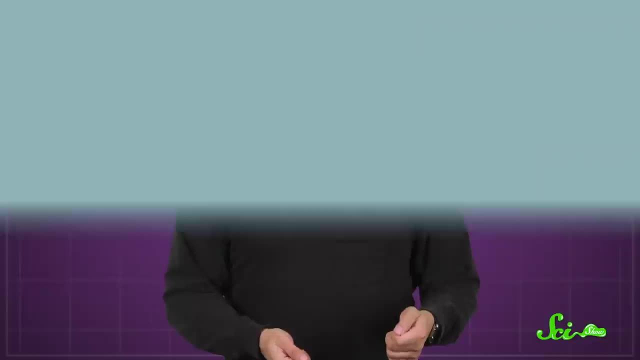 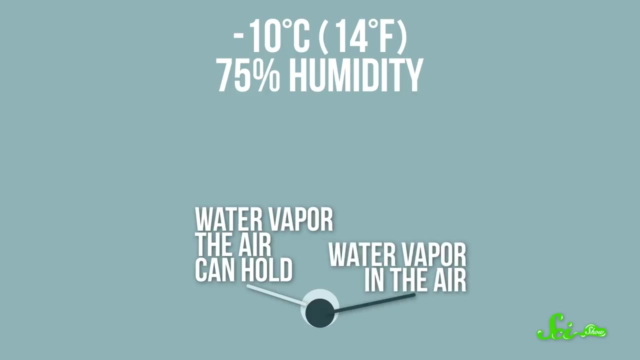 and it's why this stat usually isn't that useful in planning your day. If it's negative 10 degrees Celsius, the air can't hold as much moisture, so 75% humidity isn't actually that humid. But if it's 20 degrees, 75% humidity suddenly means. 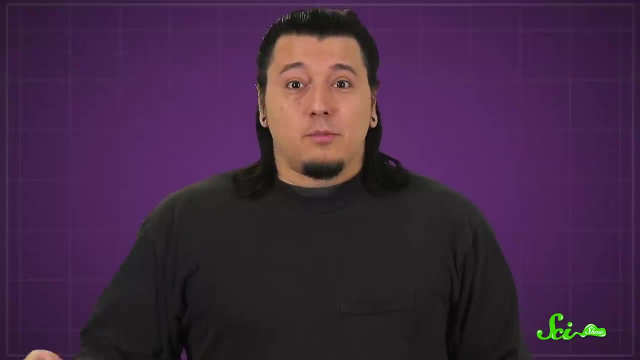 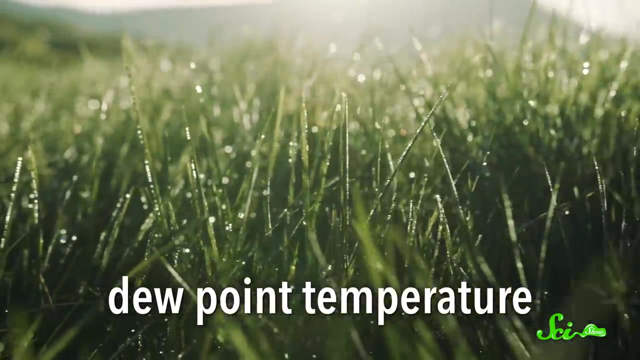 there's a lot more water in the air to make things feel all muggy. If you want a number for humidity that isn't quite so relative, try the dew point temperature. This is the temperature at which water droplets or dew form on things like grass. 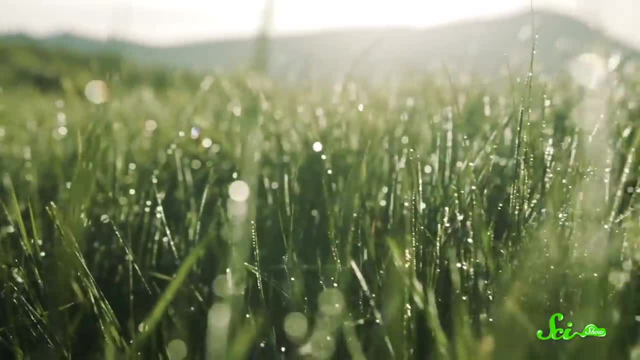 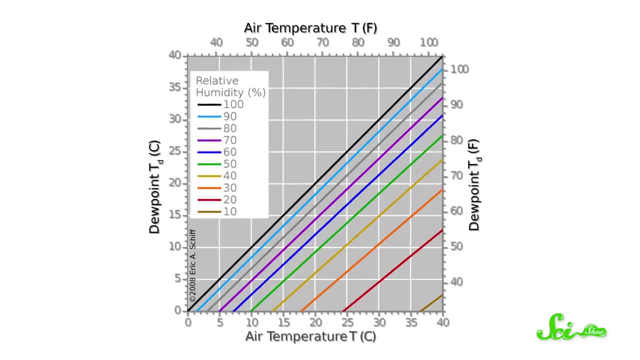 In other words, it's the temperature at which the air is completely saturated with moisture, And the closer the dew point temperature is to the temperature out here, the more humidity you get, The stickier and more unpleasant it'll be. For reference, people react differently to dew points. 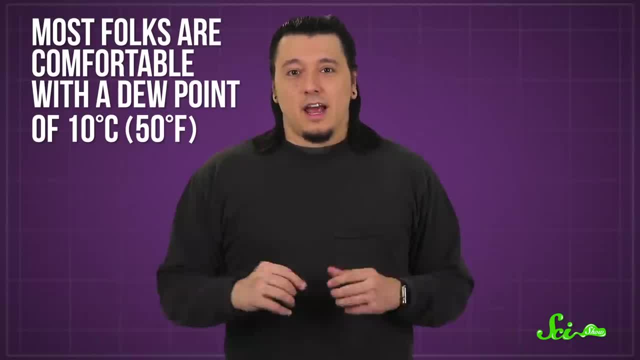 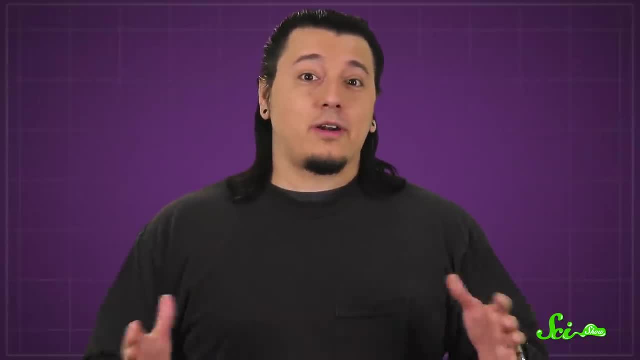 but most folks are comfortable with a dew point of 10 degrees Celsius And things get pretty humid and unpleasant around 15 to 21 degrees. So it's still a new scale to learn, but it's also consistent, no matter how cold it is outside. 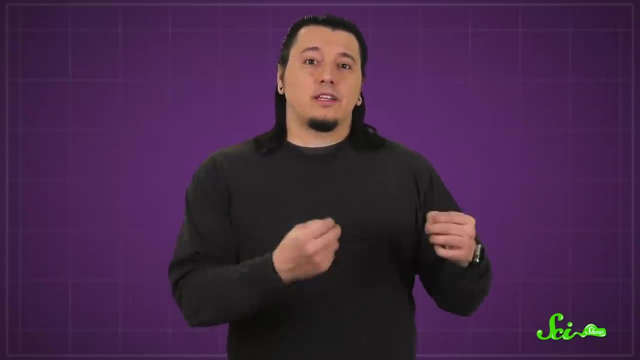 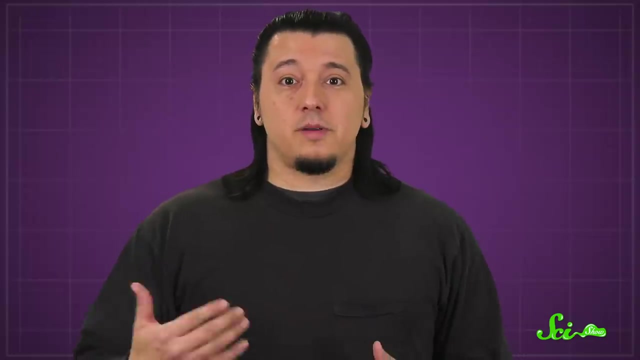 Now the big question is: if the dew point temperature is a great way to tell you how the outside world feels, why don't weather apps and weather channels use it? It's mostly a matter of history. Instruments that measure relative humidity don't always meet the ones that measure dew points. 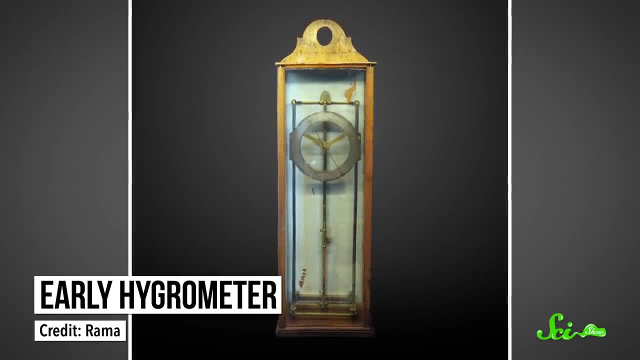 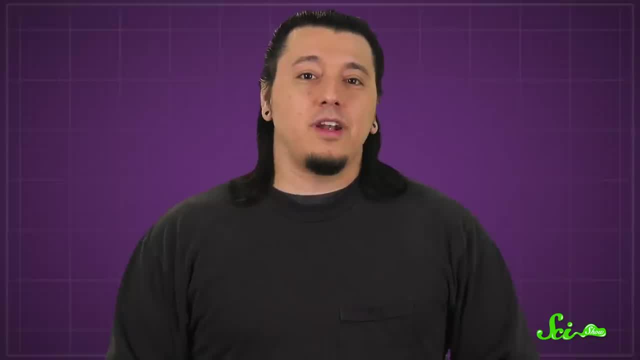 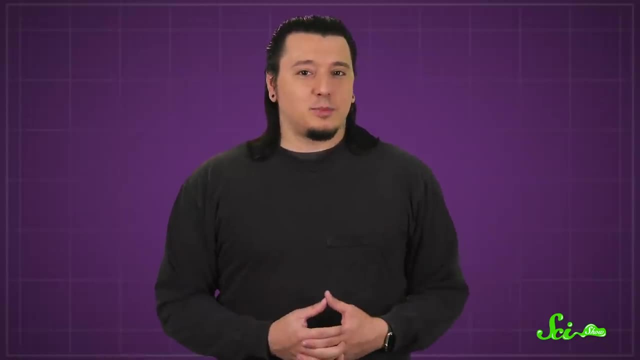 Like one of the first mechanical hygrometers, a device that measures humidity appeared in 1783. And since these devices were widely available to the public and gave reliable measurements of relative humidity, the term unfortunately stuck around. You know what else is available to the public and gives reliable science inspiration. 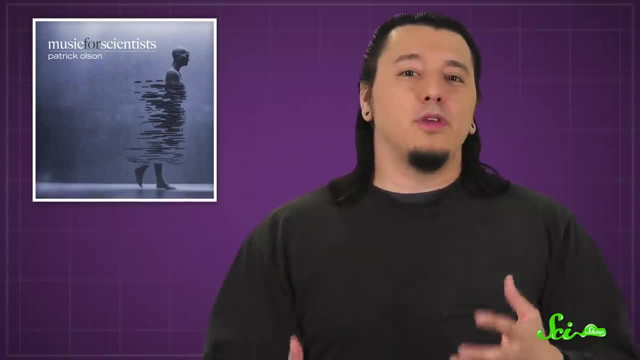 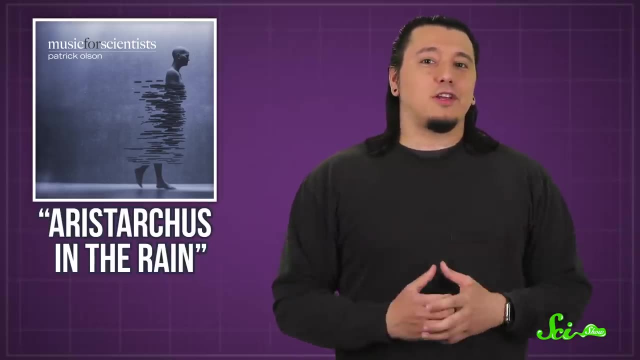 Music for Scientists, a tribute album to science, inspired by the beauty of science. It was written and recorded by Patrick Olson and it's still in the works today. If you want to check it out, I'd recommend starting off with the song Aristarchus in the Rain, which isn't about humidity. 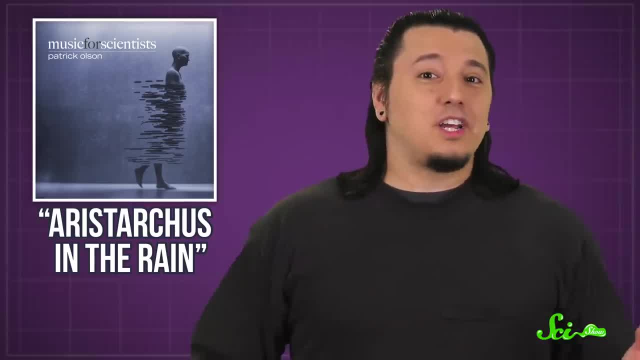 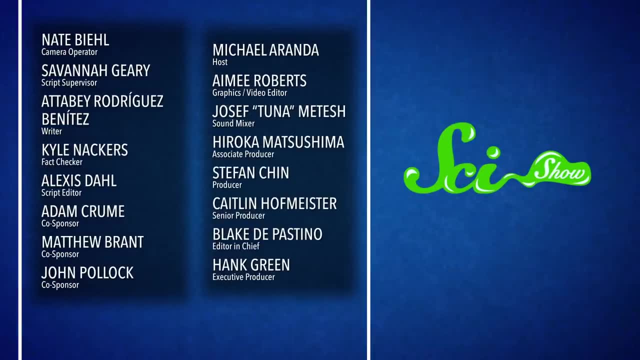 but it is about a scientist trying to make sense of this messy and cloudy world. If you want to check it out, look for Music for Scientists on all major music streaming services or click the link below. 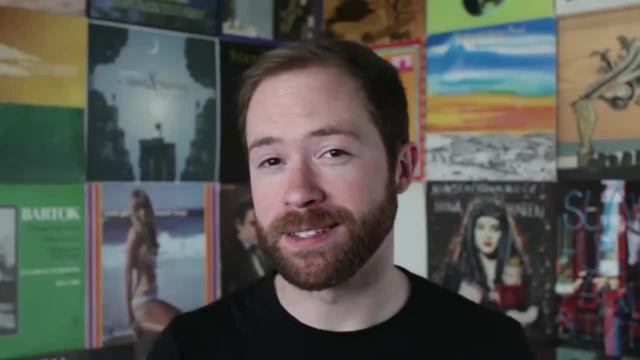 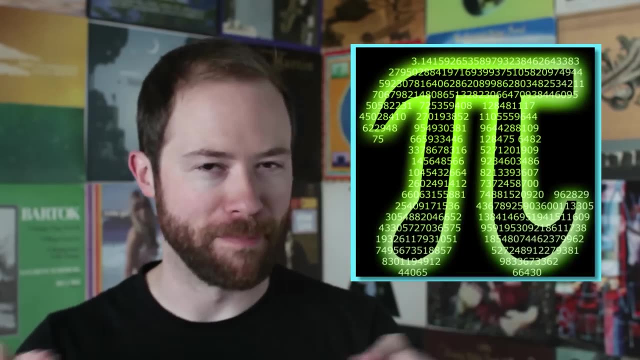 Here's an idea. Math might not actually exist. Love it or hate it, you can't argue the importance of math. Math as a system is elegant, exhaustive and frequently even beautiful. In the words of Eugene Wigner, it is quote.